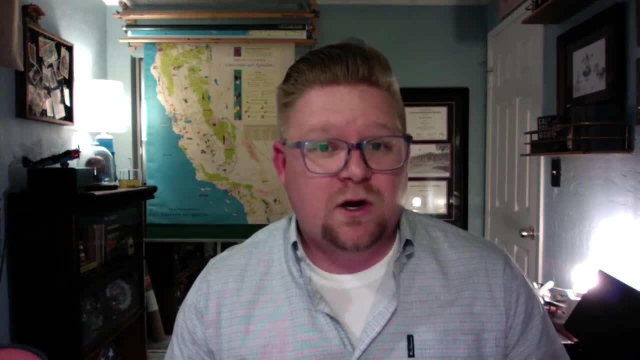 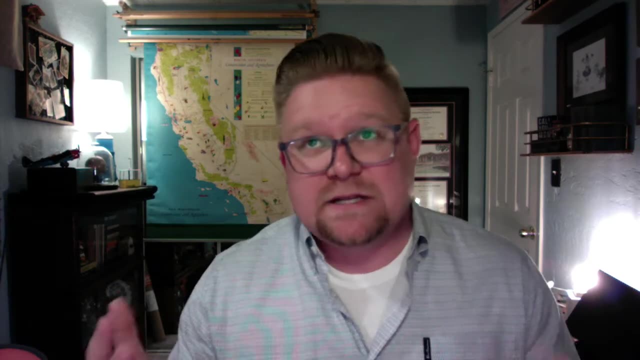 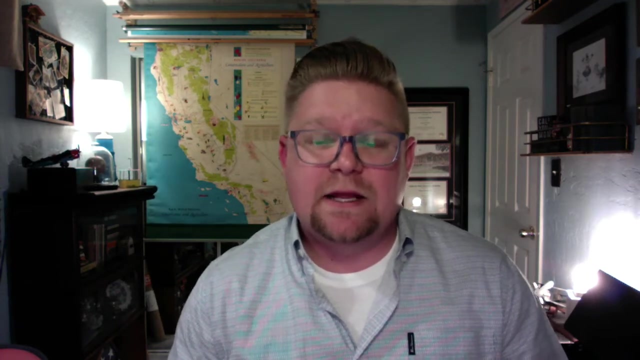 The civil war in the Democratic Republic of the Congo over the control of land and resources resulted in as many as 5 million deaths, the most since World War II. Large deposits of gold and diamonds and other rare minerals, such as coltan, are located in the Democratic Republic of Congo, and 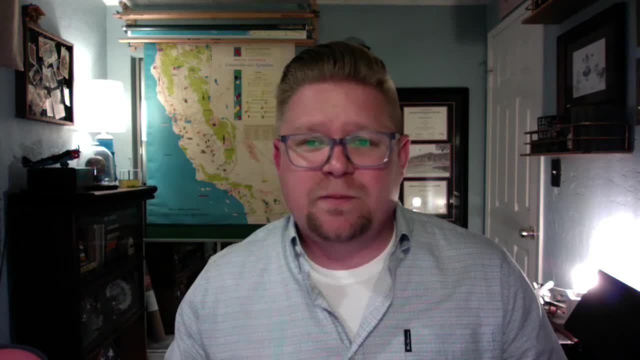 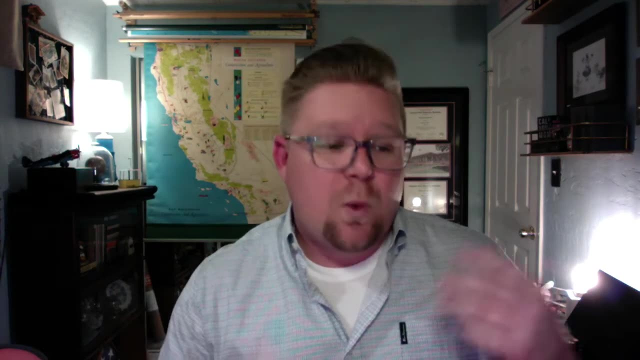 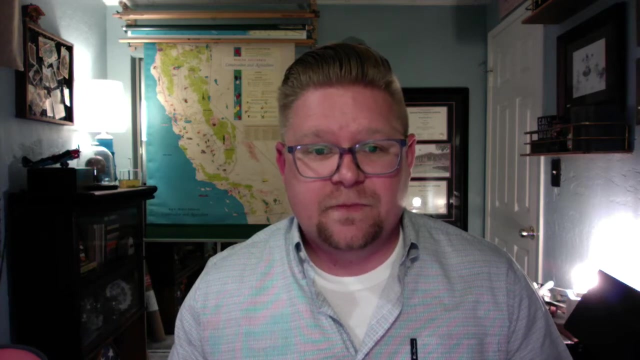 surrounding areas. The wealth they can generate has fueled many armed conflicts by various groups. Those are some things to take into consideration. within that region, Women have also suffered serious setbacks in their rights and status in the Central Africa region because of these conflicts. East Africa is dominated by the Great Rift Valley and with its 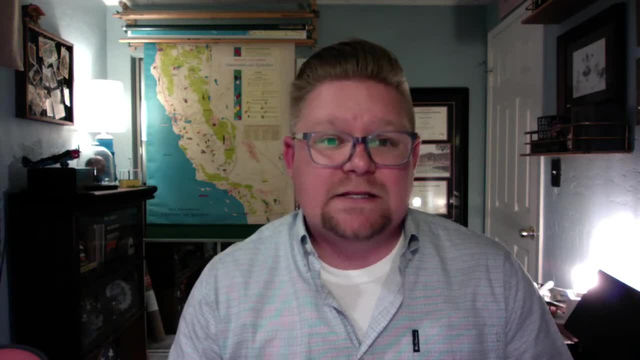 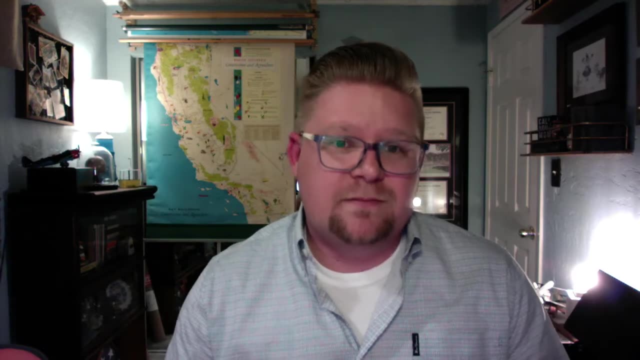 large lakes, high mountains and vast savannah plains. the Serengeti and other game preserves are home to immense numbers of big game that are attractive for tourism, but then again, most of the people that live in these regions are highly involved in agriculture. 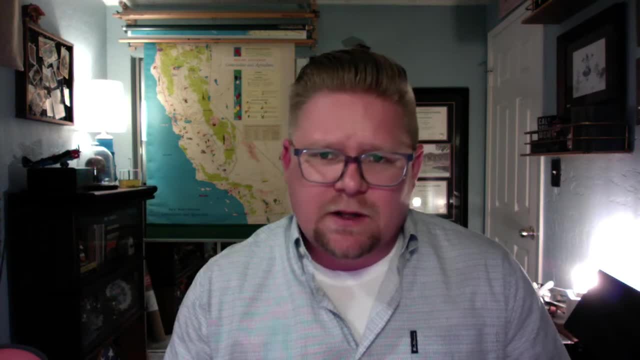 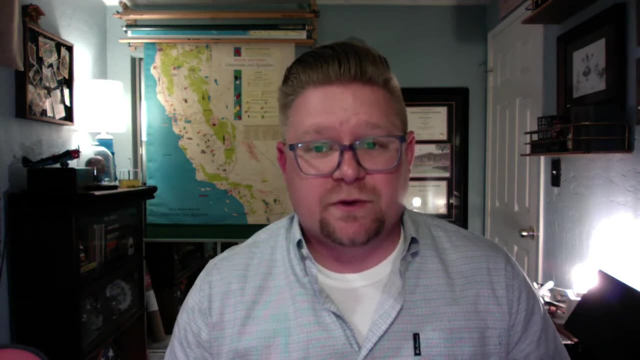 Southern Africa, located on the Tropic of Capricorn, has moderate climates, extensive mineral deposits, and the countries have a positive means to gain wealth from agriculture and these minerals. There is high diversity of tribal groups that have been impacted by colonial activity. 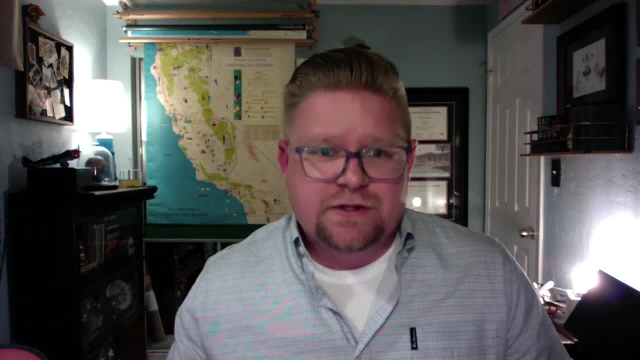 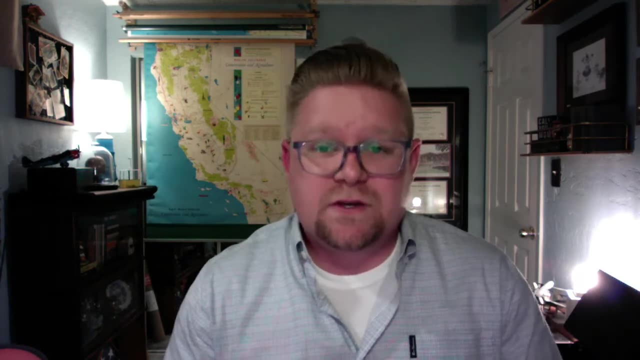 South Africa had an apartheid system and for years that eventually broke down within the last few decades Now. lastly, Madagascar is a large island off the east coast and has different flora and fauna from the mainland. South Africa is a large island off the east coast and has different flora and fauna from the mainland. 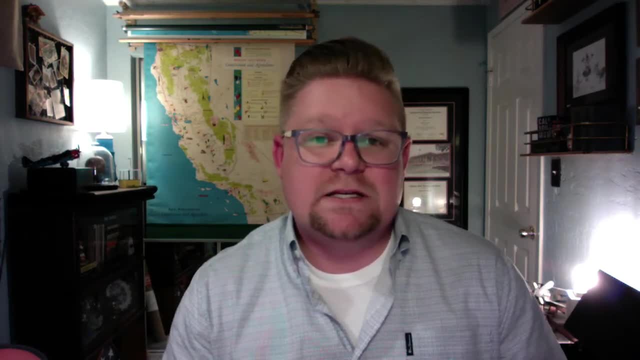 South Africa is a large island off the east coast and has different flora and fauna from the mainland, Mostly because of its isolation due to its tectonic activity. The island of Madagascar was once connected to the African continent, but drifted away with the activity of tectonic plates in that area. 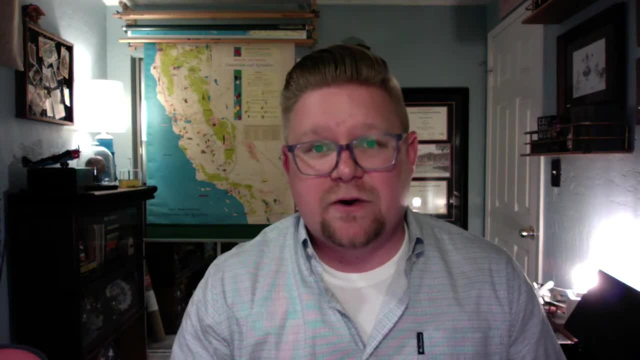 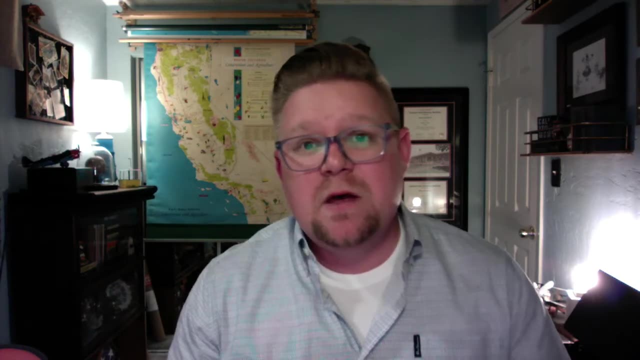 The island of Madagascar was once connected to the African continent but drifted away with the activity of tectonic plates in that area. Again, really big pieces, a lot of diversity, a lot of turmoil in these regions, Moving forward into chapter 8, which introduces the northern part of Africa and southwest Asia. 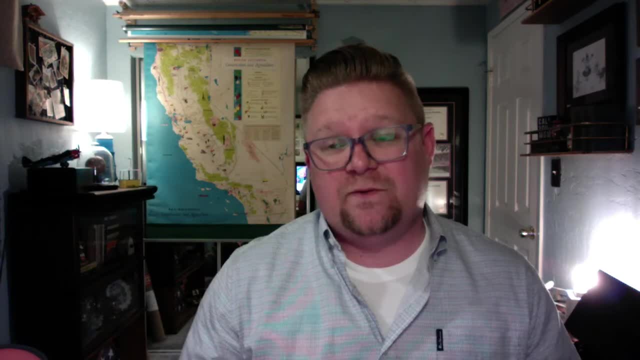 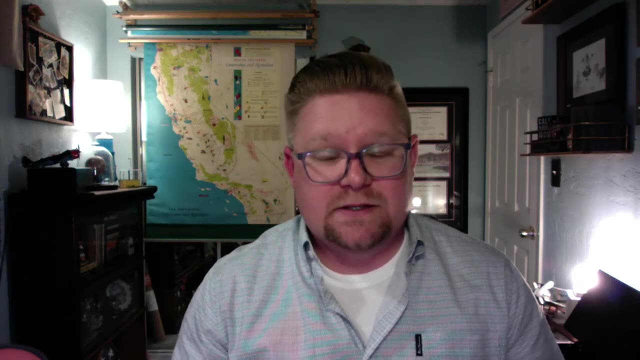 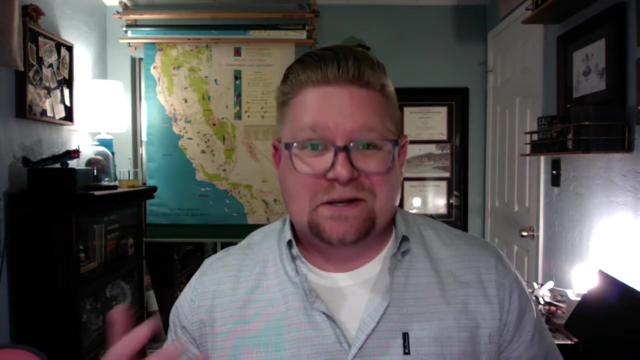 we'll see that that also continues. We'll find that really an ardent scale of progress. aside from just the differences culturally, It really has to do with natural resources. That really causes a lot of struggle and it also can cause a lot of turmoil when involved with how the politics work in those regions. 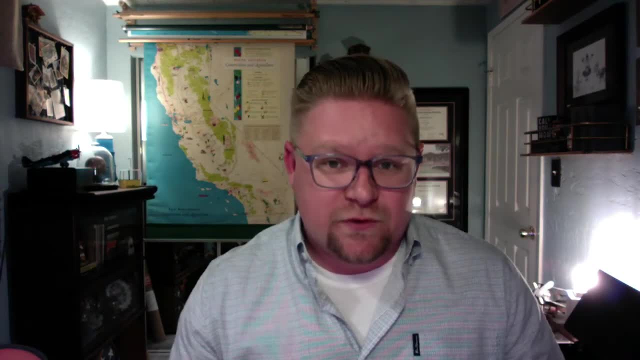 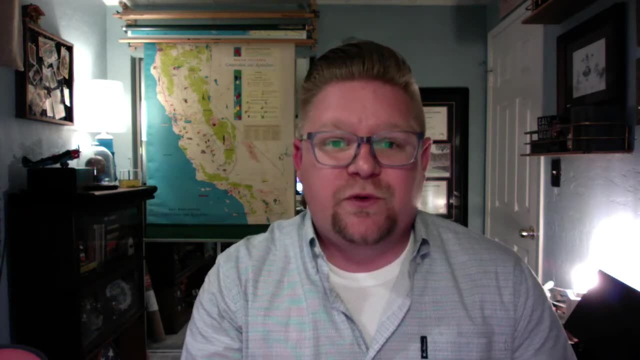 Now North Africa, Southwest Asia and Central Asia, otherwise known as Turkestan, are included in the realm of North Africa and Southwest Asia, which is dominated by the religion of Islam. This region is also arid. It's actually a bee climate. 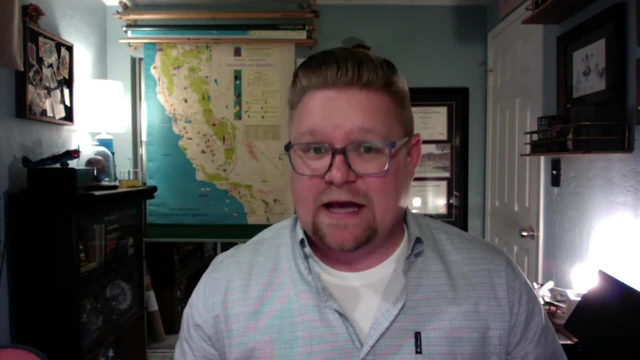 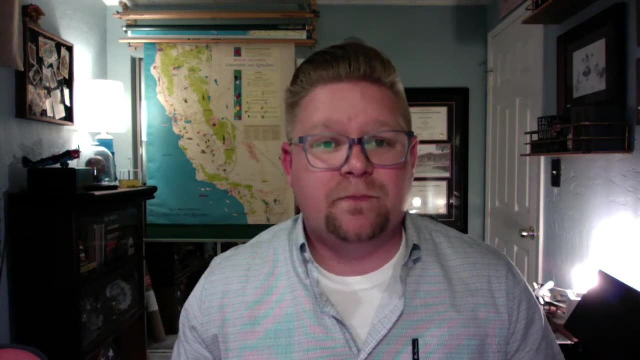 Bee, as in boy, And the export of oil and natural gas. Now, large expansive deserts make up most of the physical area of all three of these regions of the realm Water is of particular importance, as most of the population has traditionally made their living from agriculture. 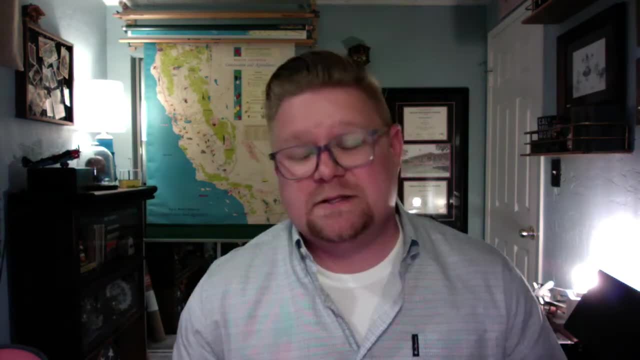 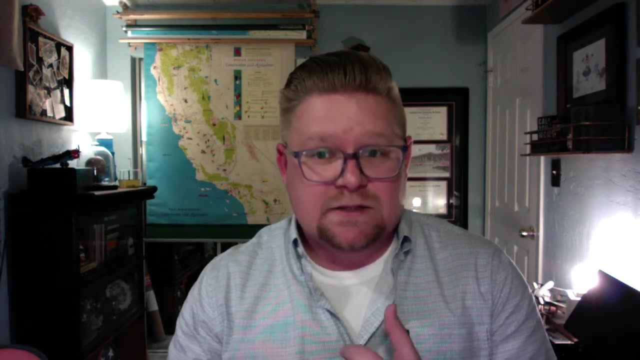 So we find that division, warfare and conflict are a constant element in these regions. Now, the three main monotheistic religions, Judaism, Christianity and Islam, all emerge from the Middle East And can be traced back to a common patriarch, Abraham. 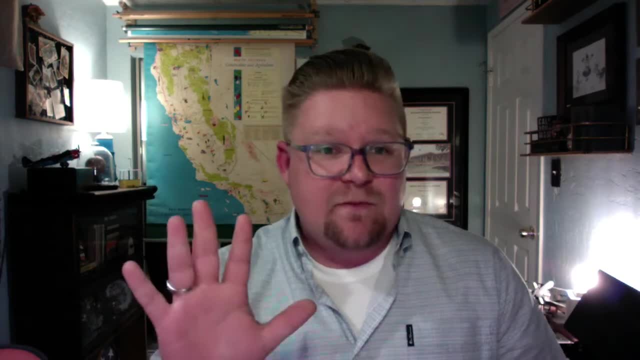 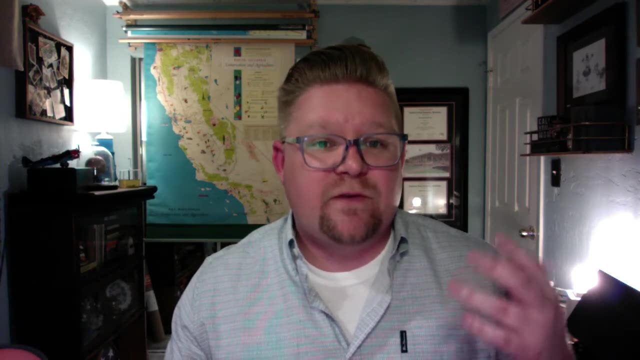 Most of the people in this realm are now Muslim. The five pillars of Islam create a guide for Muslims to live by. Mecca, the holiest city for Muslims worldwide, is where the Prophet Muhammad started the religion itself. The two main divisions of Islam are going to be Sunni and then Shia. 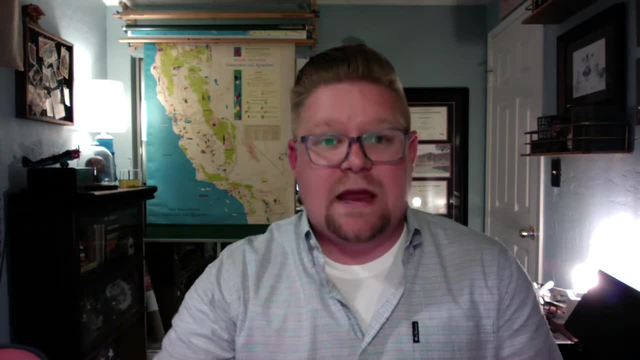 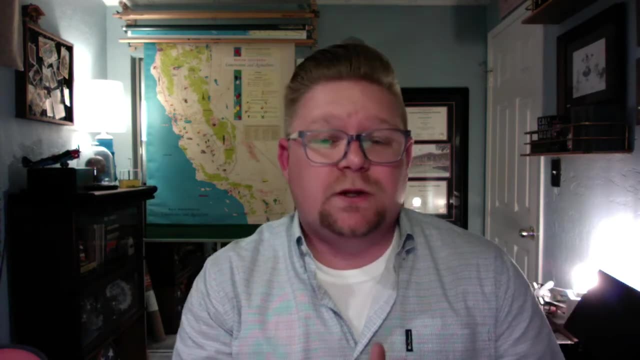 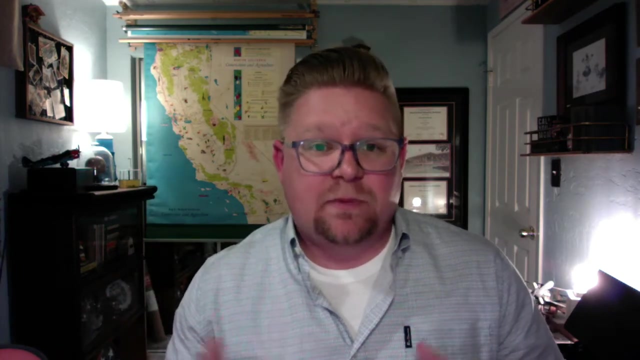 Sunni is about 84% and Shia is about 15%, And then the remaining are part of other divisions of smaller religious groups. Now North Africa includes the countries that border the Mediterranean Sea and Sudan and the Red Sea as well. Most of these people in North Africa, again, are Muslim. 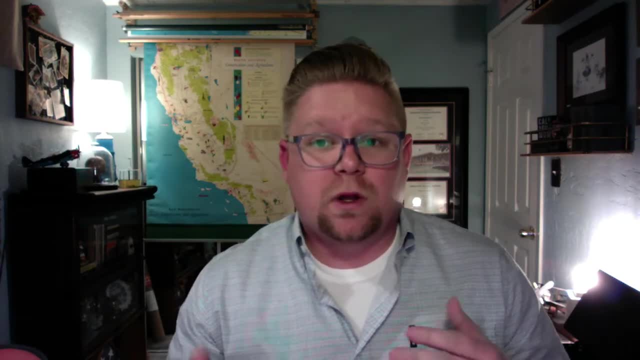 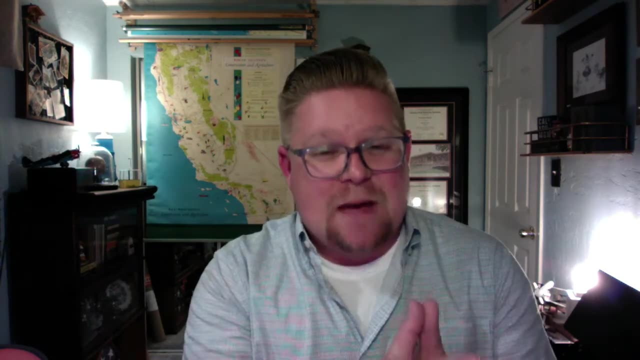 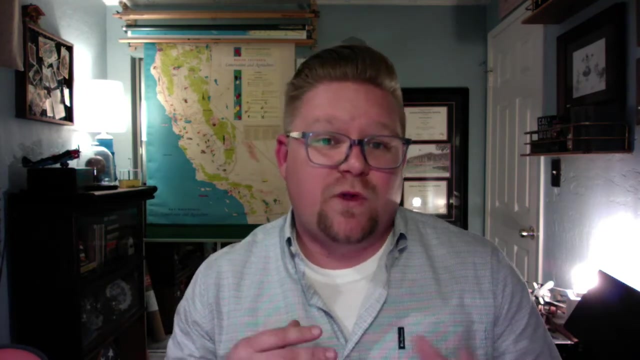 The high population areas are along the coast or along the Nile River. The Atlas Mountains trap moisture, which then provides precipitation for agriculture within the mountain valleys themselves. The countries of North Africa have all witnessed political uprisings in which the people have demanded democratic reform and increased civil rights. 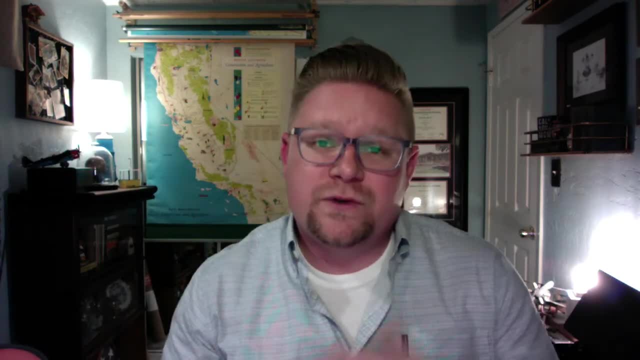 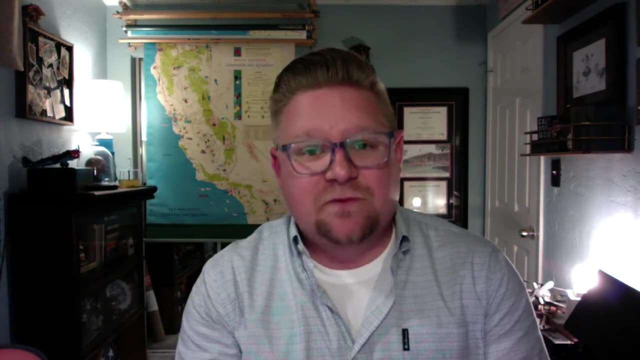 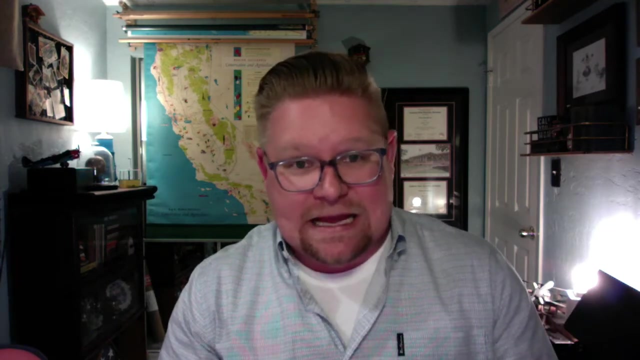 Egypt is the most populous Arab country and the cornerstone of the Arab world Moving forward. Palestine was divided in half in 1945 into the Arab state and the Jewish state. The Jewish state became the nation of Israel in 1948. Since that time, there has been constant struggle. 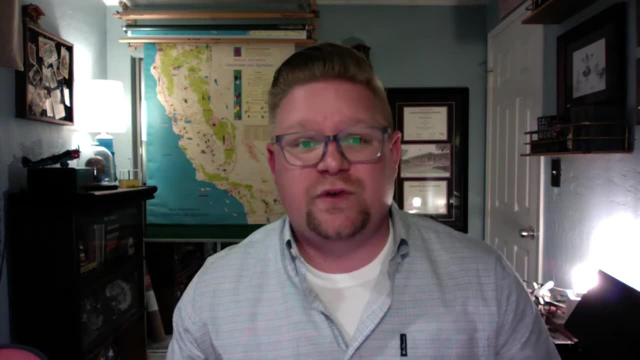 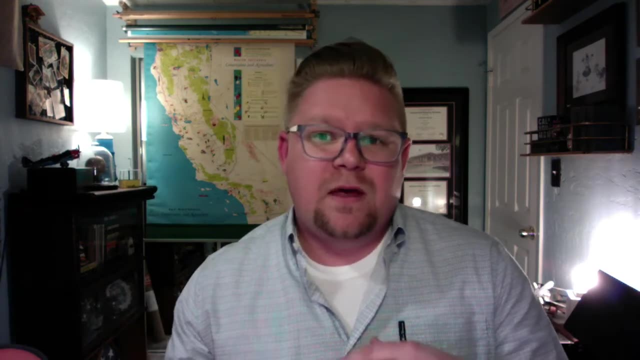 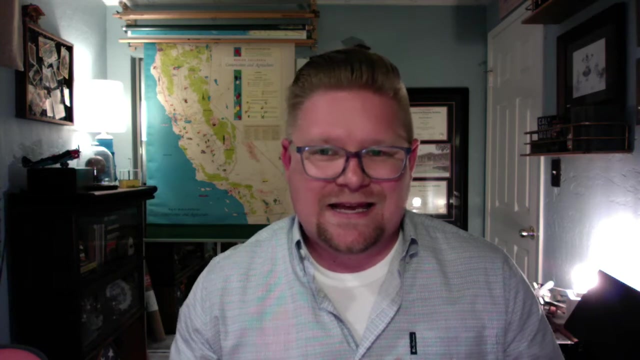 between the mainly Arab Palestinians and the Jewish state of Israel. The West Bank and the Gaza Strip are Palestinian regions that have worked to be recognized with equal sovereignty. The solution to this division is debated. Both sides have claims that they are incompatible with each other. 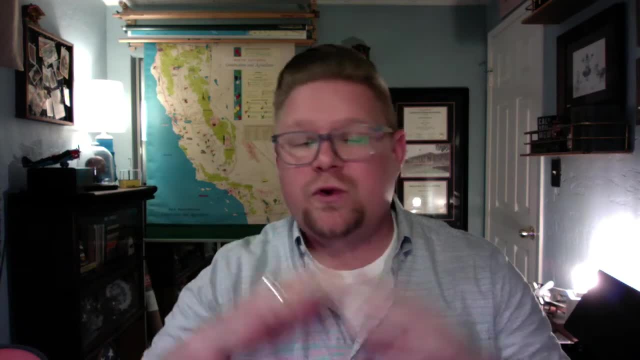 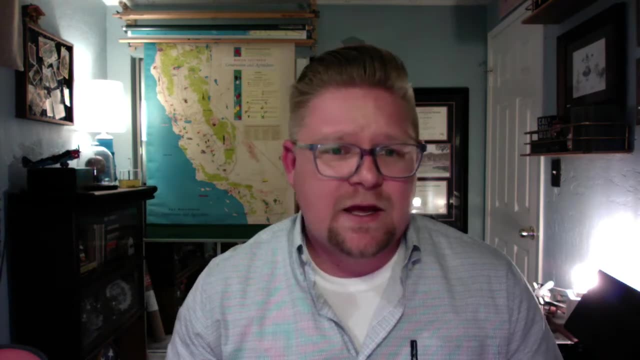 The neighboring Arab states of Jordan, Syria and Lebanon have their own unique political situations as well. Moving forward within this, we see that Iraq was the center of the Fertile Crescent of Mesopotamia, which is the center of the Fertile Crescent of Mesopotamia. 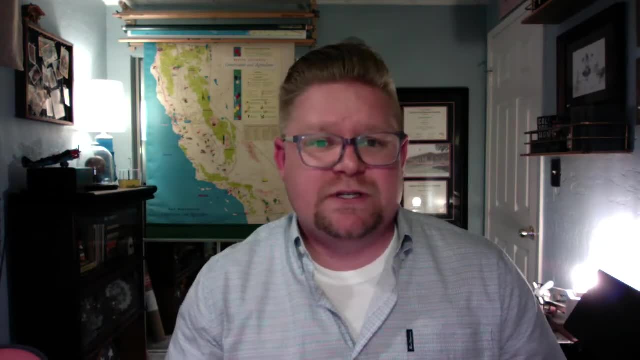 the center of the Fertile Crescent of Mesopotamia, the center of the Fertile Crescent of Mesopotamia, which is the center of the Fertile Crescent of Mesopotamia, which spawned early human civilizations. The country is divided between Shia majority and Sunni minority. 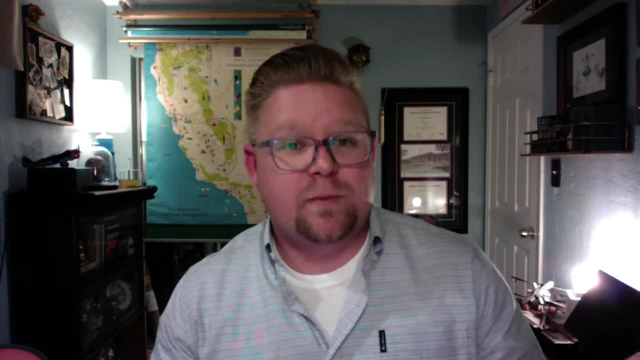 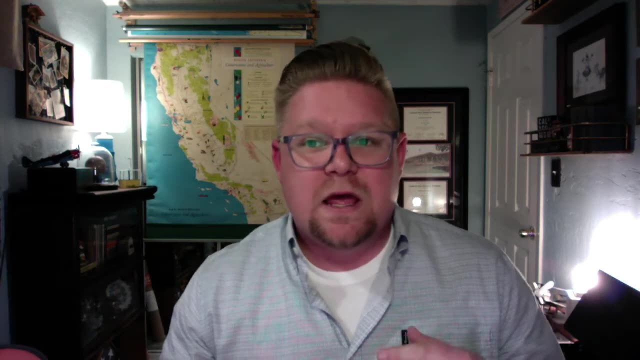 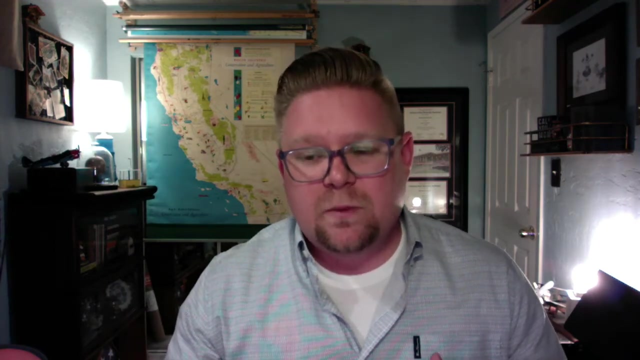 It is also an Arab country with a large minority group of Kurds. to the north, Iraq has enormous oil reserves that have not yet been developed for exploitation, which has attracted the attention of the world's energy-dependent core regions. We will discuss further within the book, as you'll see. 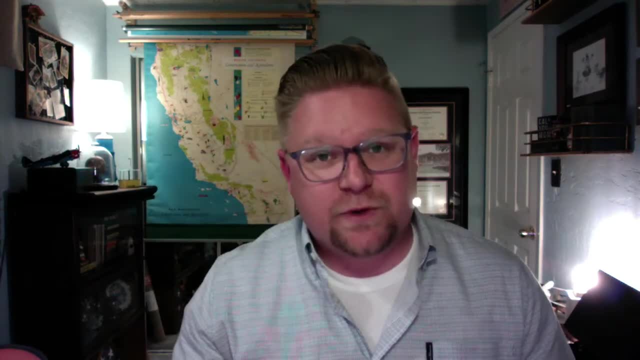 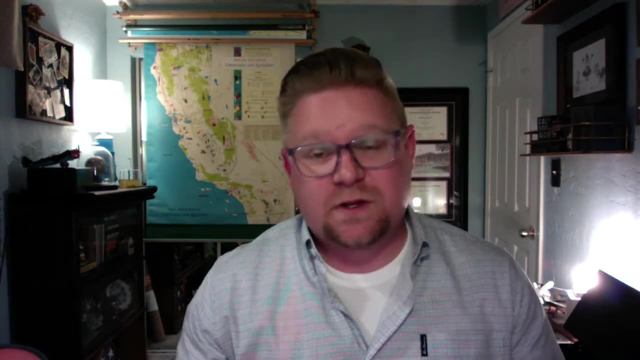 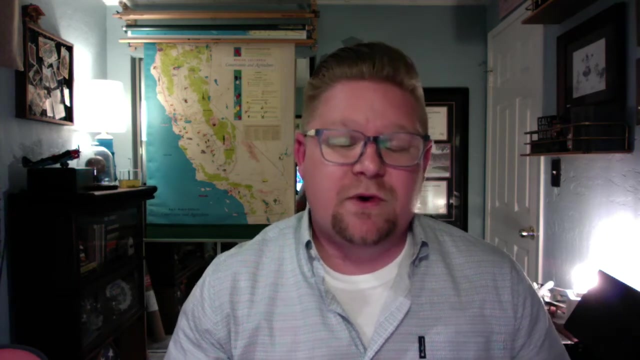 about these both natural and unnatural resources for power. There has been discussion not only that about 25% of the world's oil is found within these regions, but there also, if you think about it, because of where the tropics lie and the fact that it's very dry in most of these areas. 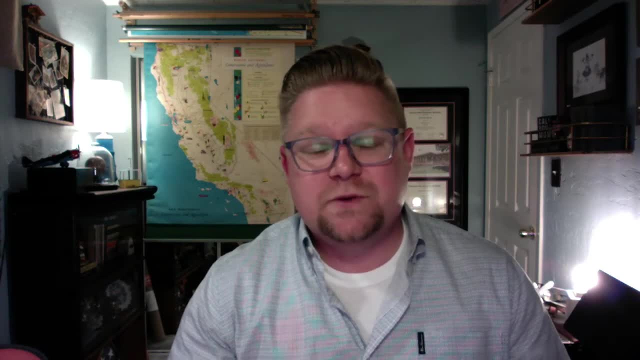 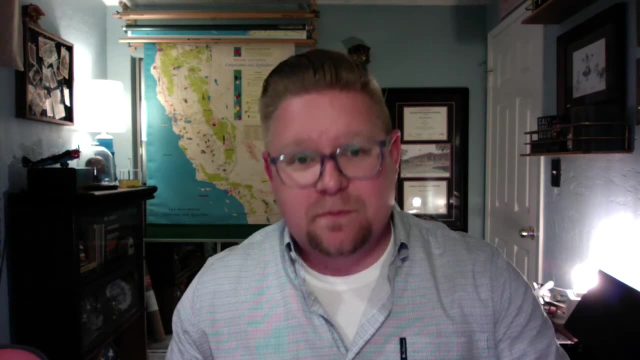 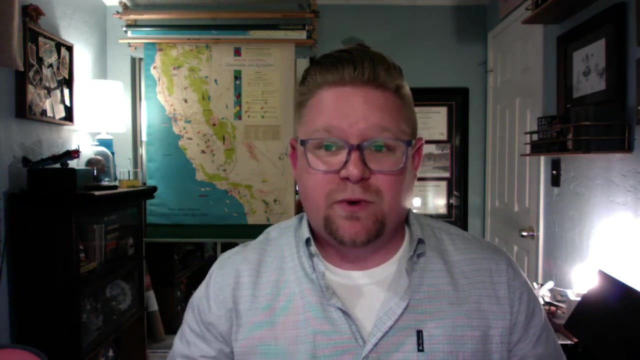 that it's actually one of the best places for solar energy as well, So it's really kind of the hub for that type of energy piece. So last bit of this We'll mention is that Afghanistan has been conquered by many empires and was a buffer state between British and Russian colonial efforts. 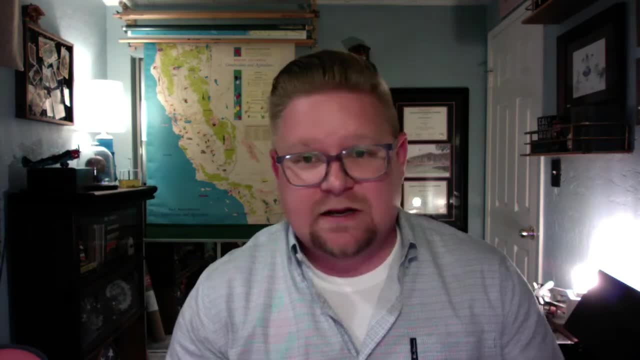 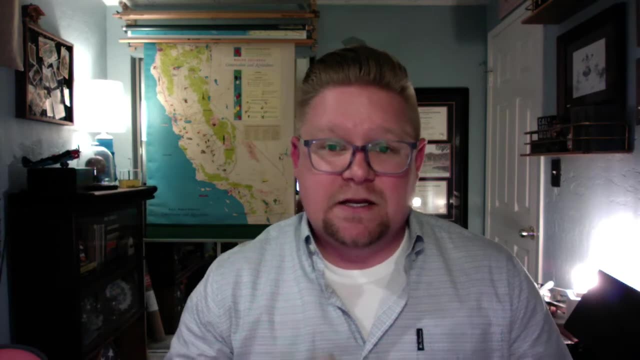 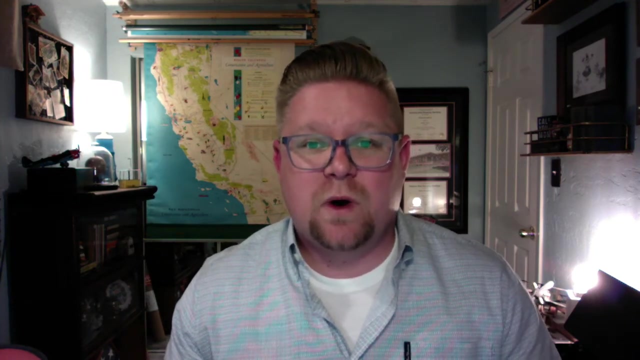 The country has a dry, rugged terrain and a devastated economy. The people are very poor, with very little infrastructure, The many tribal groups that made it difficult for a centralized government to be effective. The United States invaded Afghanistan in 2001 to remove al-Qaeda training camps run by Osama bin Laden. 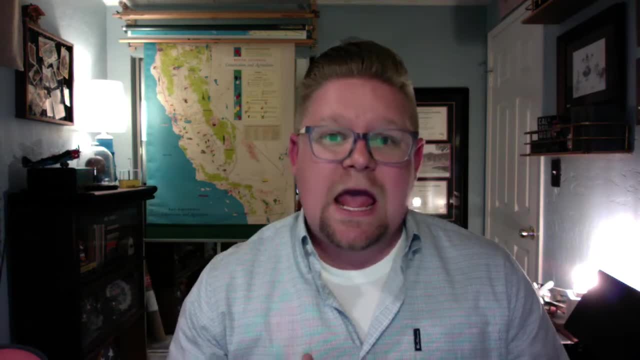 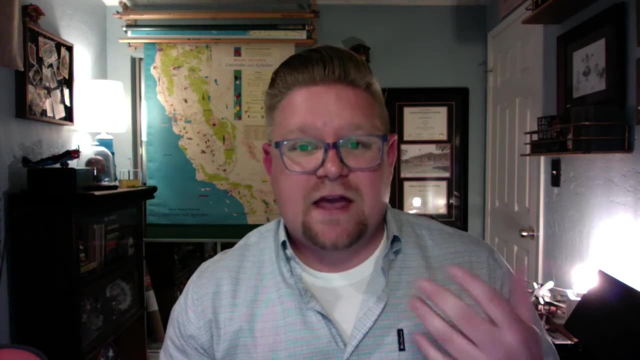 Now the United States has a very poor infrastructure. The North Atlantic Treaty Organization, or NATO, forces have taken over the mission in Afghanistan to defeat the Taliban extremists and support stability for the country. Afghanistan has enormous amounts of mineral resources that are in high demand by the world's core industrial regions.